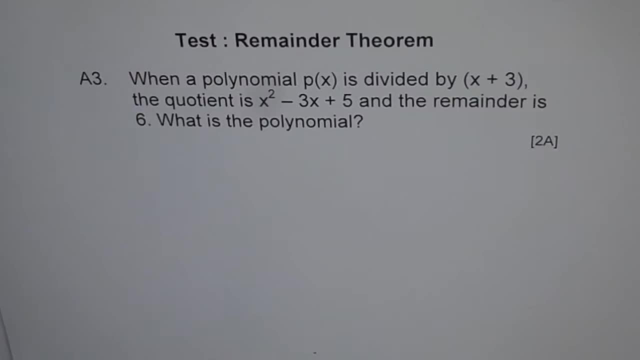 Here we have an application problem from remainder theorem. Well, actually I should say division statement A3.. When a polynomial P of x is divided by x plus 3, the quotient is x squared minus 3x plus 5 and the remainder is 6.. What is the polynomial? 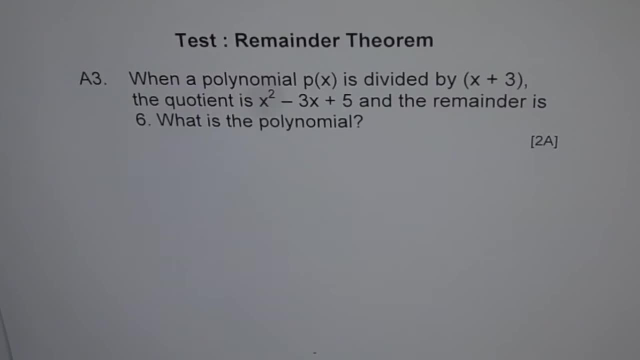 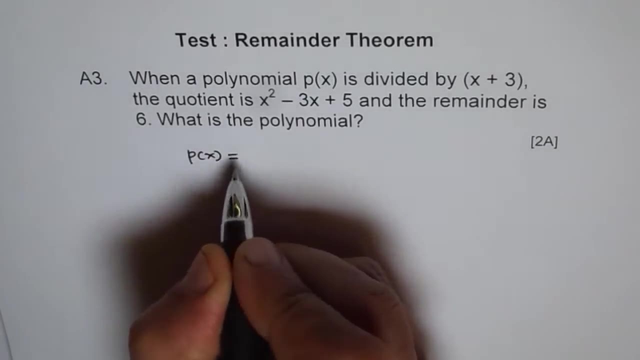 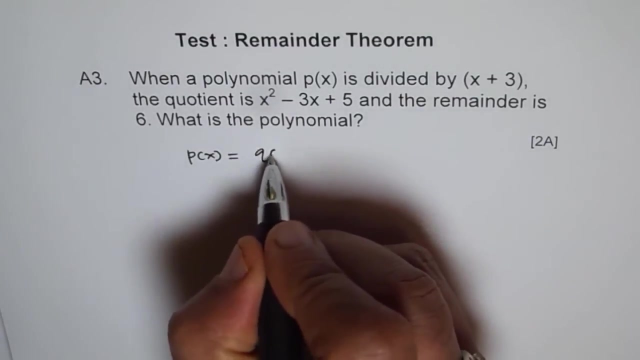 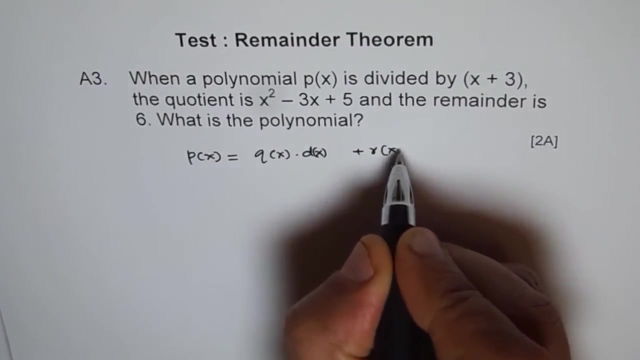 Okay Now I hope you remember the division statement right. From the division statement we can say: polynomial Px is equal to quotient times divisor right Plus remainder correct. So that's the division statement, right. We need to find polynomial. 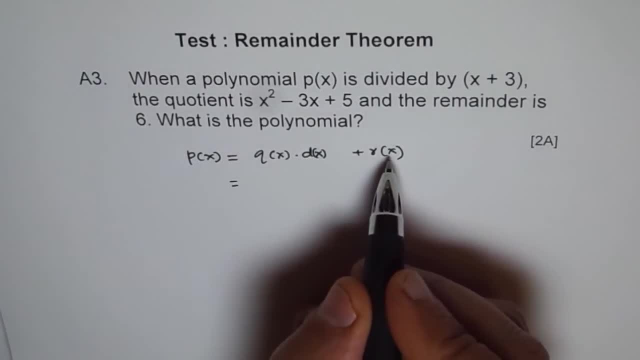 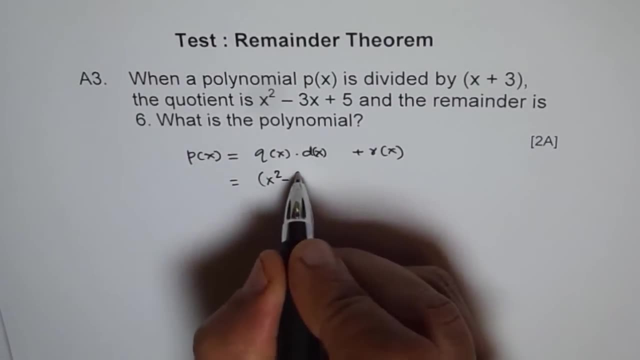 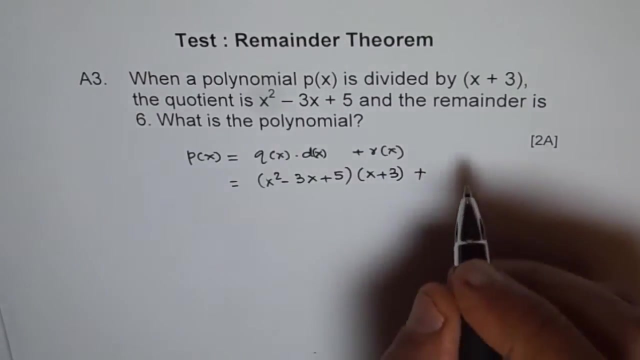 Okay, And we are given quotient, divisor and remainder. So let's do it. Quotient is x squared minus 3x plus 5. Divisor is x plus 3. Plus remainder is 6.. That's it. 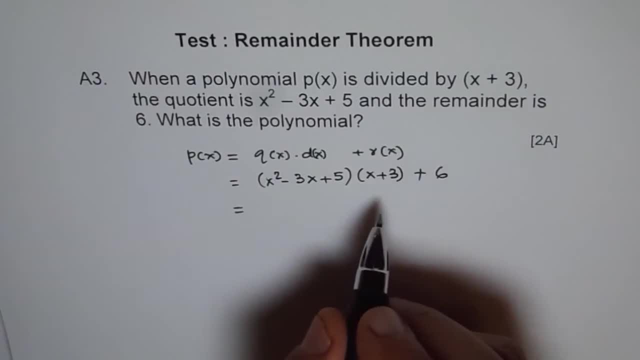 And if we expand it and combine the like terms, you should get your answer. So x times x squared is x cubed minus 3x squared plus 5x. And now with 3, right, 3x squared minus 9x. 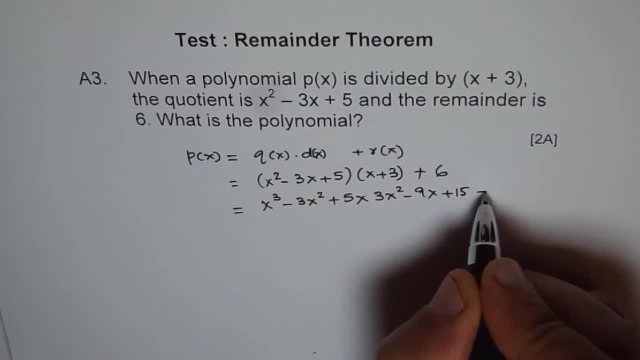 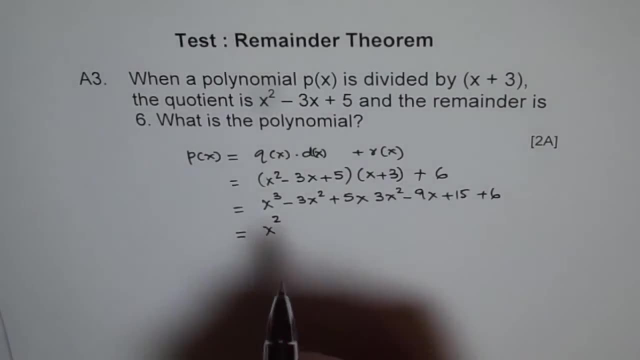 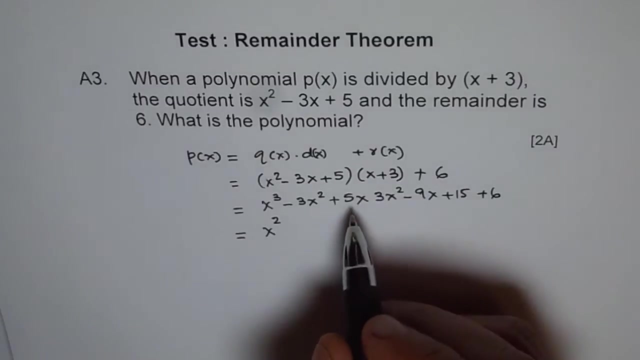 plus 15 plus 6.. Let's combine the like terms and we get x squared minus 3x squared. and what happened here? So we had 5x. Here we have 5x and plus 3x squared, plus in between, correct? 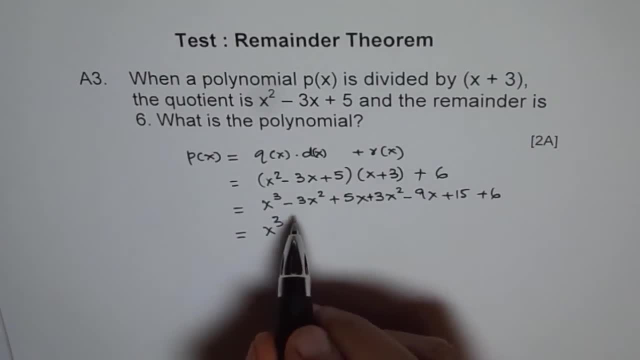 So we have 3x cubed, and then we have minus 3x squared plus 3x squared is 0, and 5x n minus. so we get minus 4x and 15 plus 6 is 21,, right. 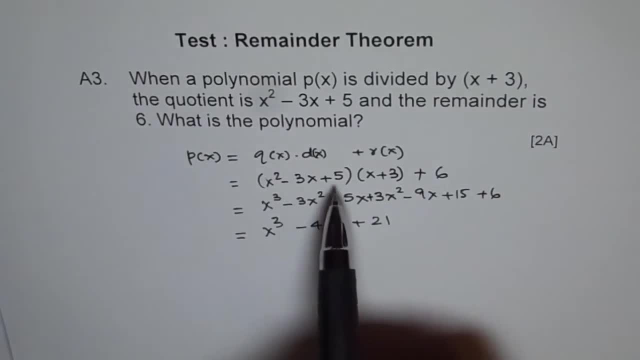 Let's check it: x squared minus 3x plus 5 times x plus 3 plus 6, x cubed minus 3x squared plus 5x plus 3x squared minus 9x and 15 plus 6..